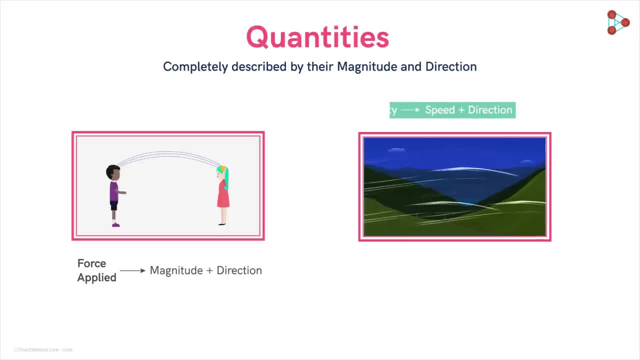 The speed of an object, along with the direction it's moving in, is called its velocity. So here we can say that the velocity of the wind at this place is 30 kilometres per hour in the north-east direction. This means that the magnitude of the wind's velocity is 30 kilometres per hour. 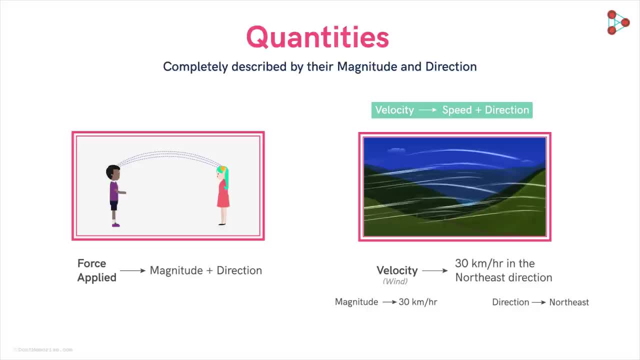 and its direction is north-east. Such quantities, which are completely described by its magnitude and its direction, are called VECTOR QUANTITIES. In mathematics and physics, you will encounter many vector quantities like this. Some more examples of vector quantities are: displacement, acceleration. 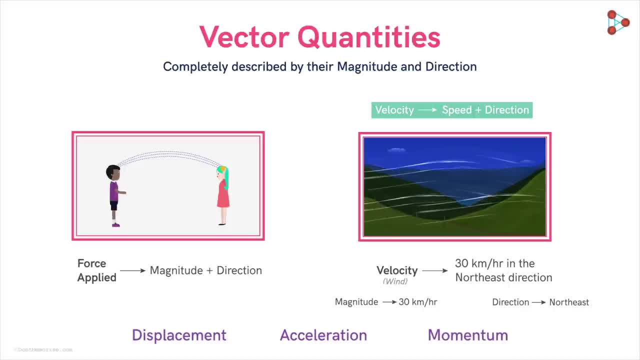 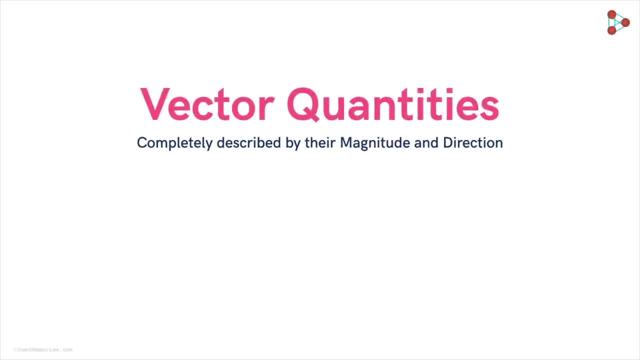 momentum and so on. In this video and the upcoming ones, we will understand mathematically what VECTOR QUANTITIES are. We will understand some basic concepts about VECTORS, various operations on VECTORS and their ALGEBRIC and GEOMETRIC PROPERTIES. 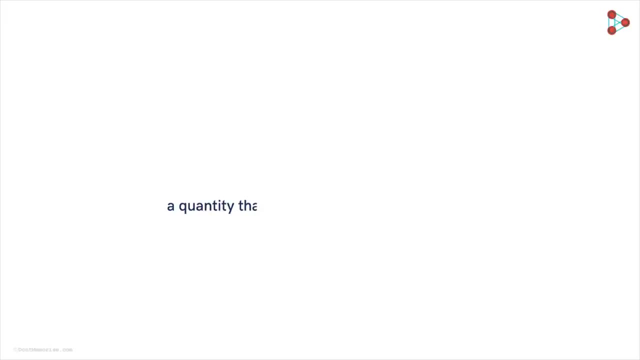 So let's get started. Mathematically, a quantity that has magnitude as well as direction is called a VECTOR. Let's consider one abstract example of it. Tell me: is a line segment a VECTOR? No right. A line segment has only magnitude, ie length, but no direction. 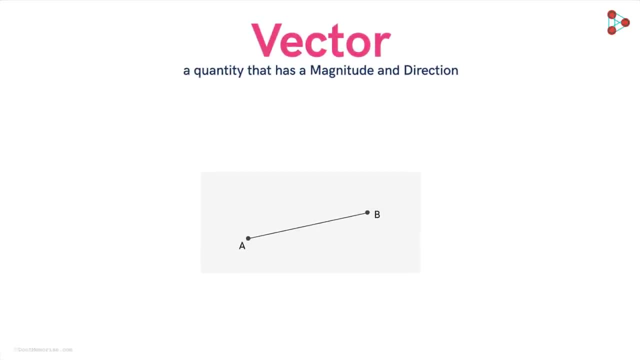 Now let's say we specify a direction for this line segment by an arrowhead. This means that the line segment is now directed from A to B, So let's call it a directed line segment. So now we have a magnitude and a direction for this directed line segment. 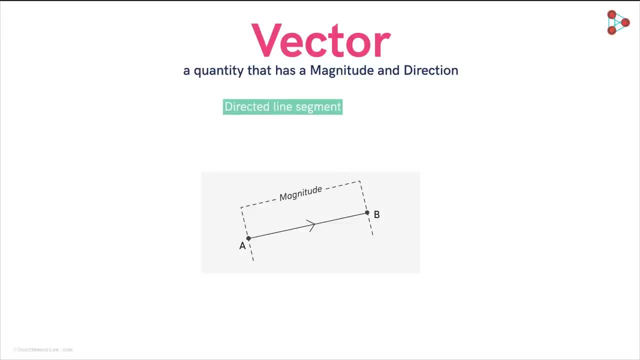 Therefore we can say that the directed line segment is a VECTOR. We denote it as this. It's called VECTOR AB. The arrow above the letters tells us that they represent a VECTOR. The point A, from where the VECTOR AB starts, is called its INITIAL point. 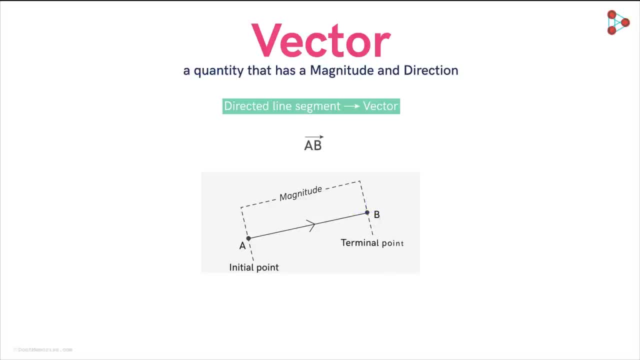 and the point B, where it ends, is called its TERMINAL point. The distance between the INITIAL and the TERMINAL points of a VECTOR is called the MAGNITUDE or the LENGTH of the VECTOR. It's denoted as this And the arrowhead indicates the DIRECTION of the VECTOR. 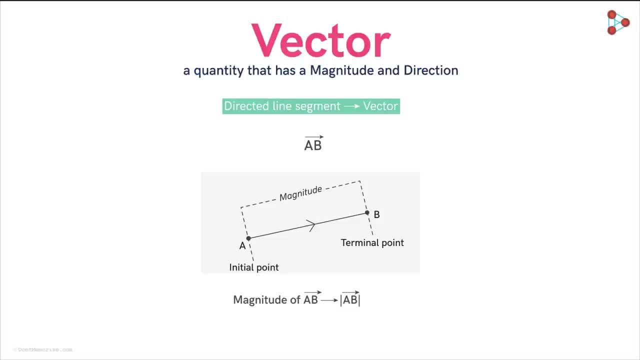 We know that for a line segment, we can show the direction in two ways. So here, instead of this, if we draw an arrowhead like this, then we can say that the line segment is directed for B to A, And thus we get another VECTOR BA. 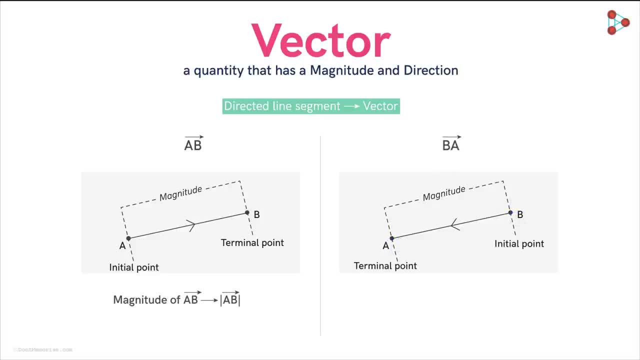 whose INITIAL point is B and the TERMINAL point is A. It has the same magnitude as VECTOR AB, but is directed in the opposite direction. Usually, to denote a VECTOR, we also use one more notation. Instead of this, we can denote a VECTOR by a lower case letter. 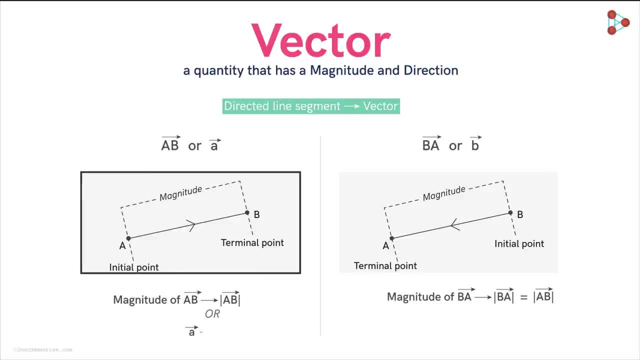 with an arrow above it. So this is a VECTOR A with magnitude denoted as this, and this is VECTOR B with magnitude denoted as this. Does we see that a directed line segment, which is a simple mathematical entity, is a VECTOR? 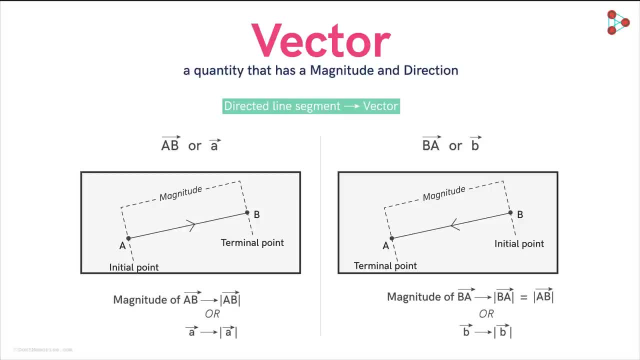 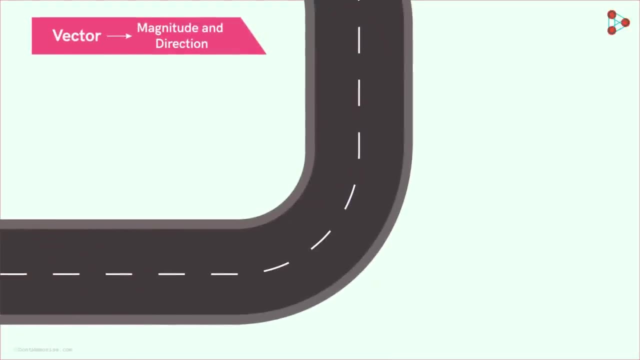 Now, to represent any VECTOR QUANTITY, we have to state its MAGNITUDE and its DIRECTION. Hence, to represent it geometrically, we usually use a directed line segment. For example, let's say that we have to represent the velocity of a car at these two places. 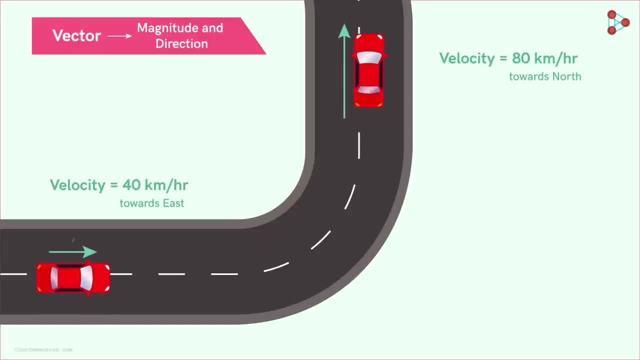 Then we represent it like this by VECTORS V1 and V2.. Now we know that the length of the line segment represents the magnitude of the vector. So as the speed here is twice than that, here we represent the length of this vector. 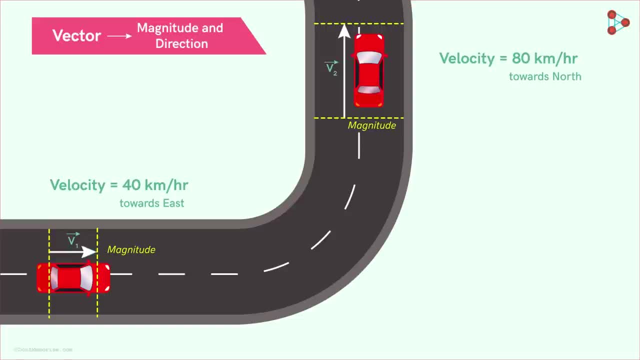 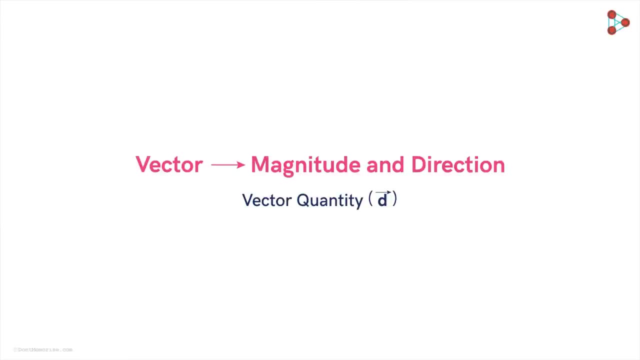 as twice the length than it's here. Does we see that if we have a VECTOR QUANTITY D, we can represent it by a directed line segment? That is an arrow like this: Its length represents the magnitude of the vector and the arrowhead its direction. 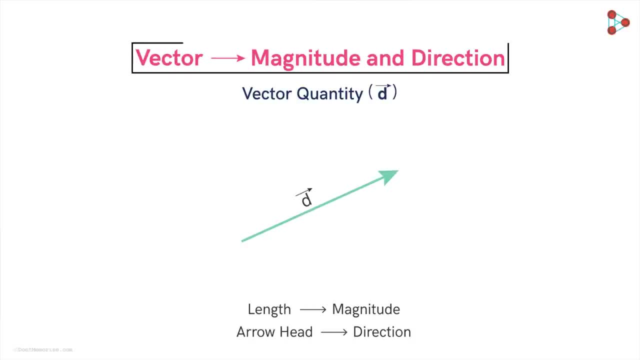 So in this video we saw what VECTORS are and how to represent them. To keep learning such interesting things, do subscribe to our channel.